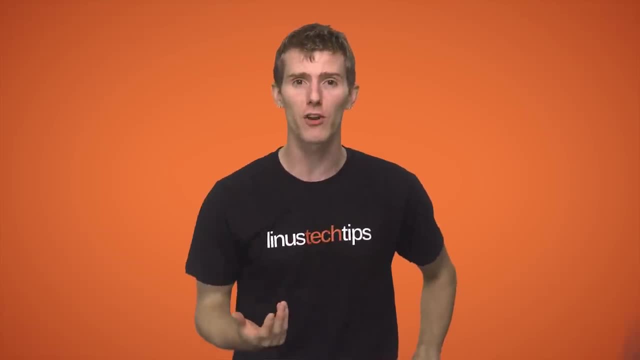 Microsoft never claims that Edge is the fastest browser on the block, So then what does it promise to deliver that other perfectly capable options don't? Great question, and we're actually going to have a full video about this on our tech wiki channel quite shortly. 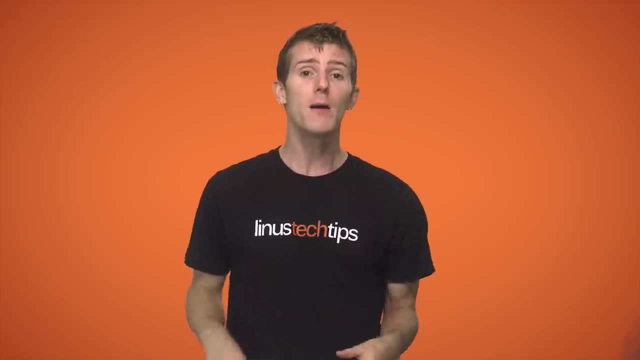 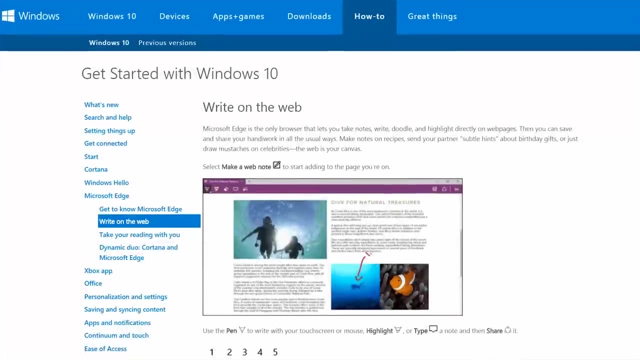 So get subscribed over there for that. But in a nutshell, Microsoft has got three main pillars for Edge. Number one is easy markup of web pages and then easy sharing. So I guess useful for Surface series tablet users and those people who are freakishly skilled at drawing with a mouse. 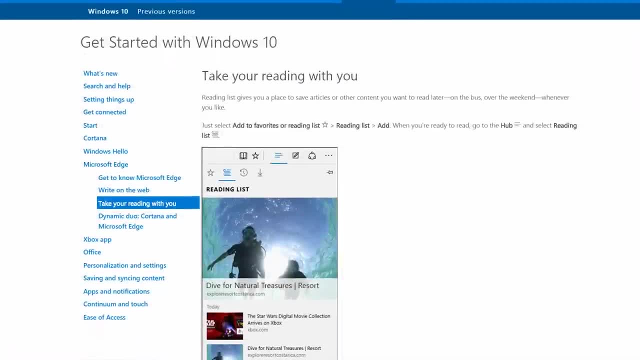 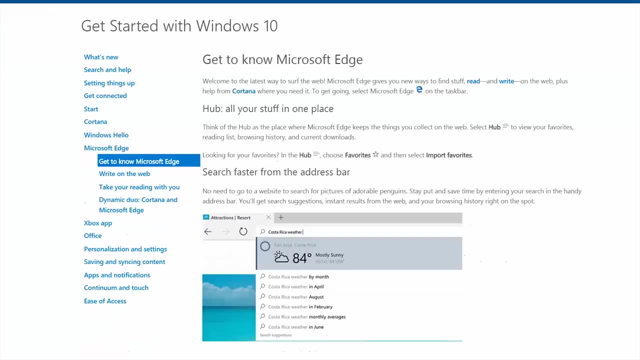 Number two is reading mode, which sweeps the unnecessary stuff out of the way and allows you to focus on what you're well reading. And number three is having Cortana as a co-pilot, who suggests stuff and delivers instant search results With Bing, unfortunately. 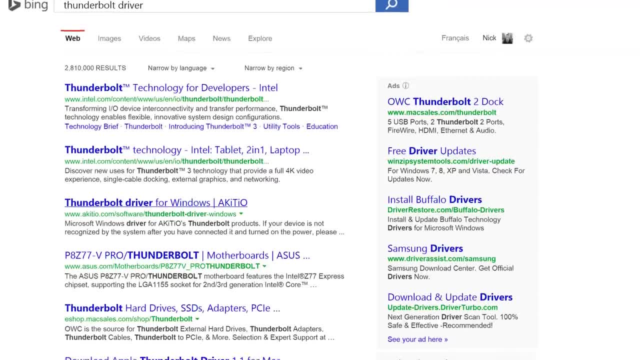 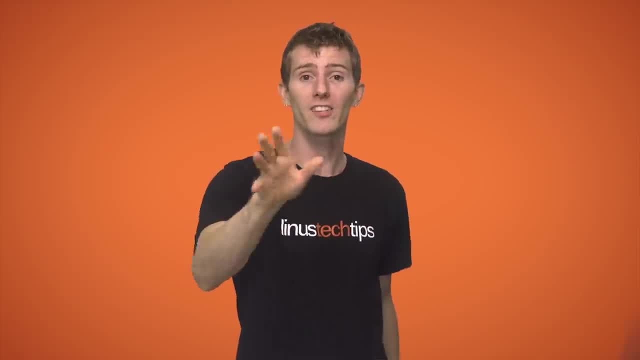 But hey, whatever Microsoft, I never wanted to actually download anything that time when I was searching for a Thunderbolt driver. anyway, Man, I hate Bing. Like how hard is this? But anyway, just like you're not tied to Edge on Windows 10, though they do make default browser switching a little more complicated than before. 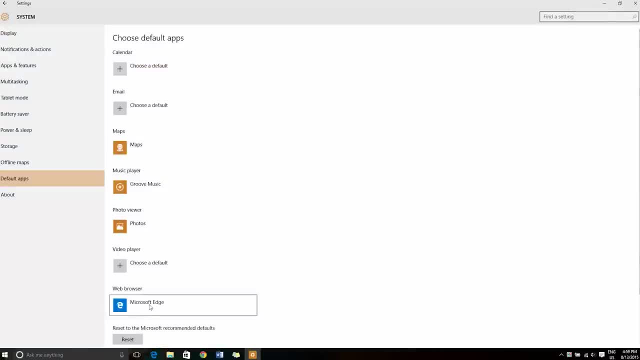 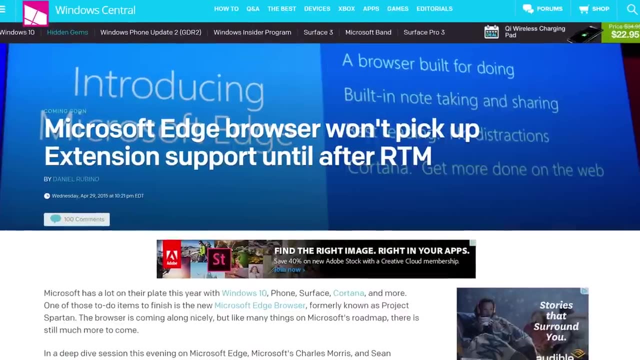 you are not tied to Bing, with Cortana in Edge if you wanted to pair her with a stronger search engine, Which I guess ties well into the unofficial but, in my opinion, super important fourth pillar. that's coming a bit later. Proper support for extensions, like the other two leading browsers from Mozilla and Google. 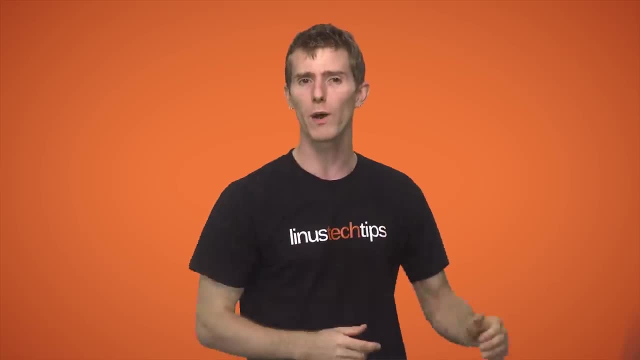 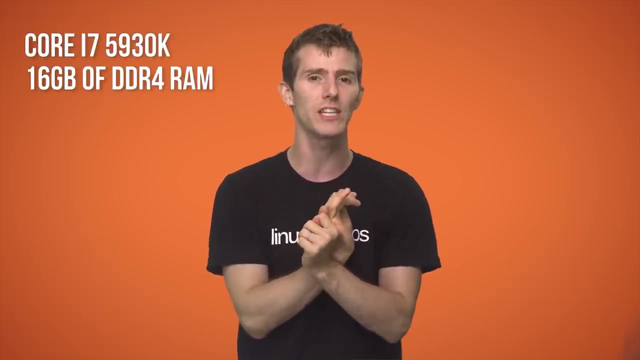 But enough of that, let's talk performance. John was the one who put together this benchmarking setup for this video and I think he did a bang up job. We used a Core i7 5930K with 16 gigs of DDR4 RAM and a Samsung 850 Pro SSD, and all tests were run on a fresh copy of Windows 10 64-bit. 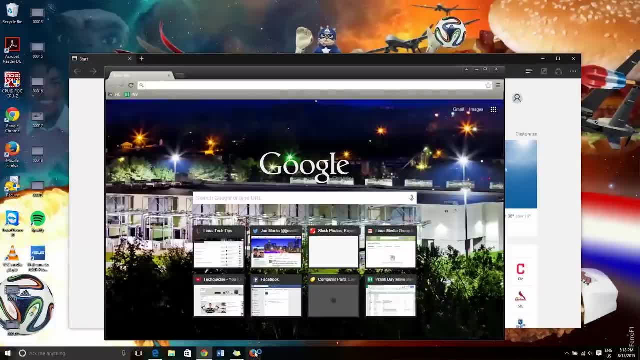 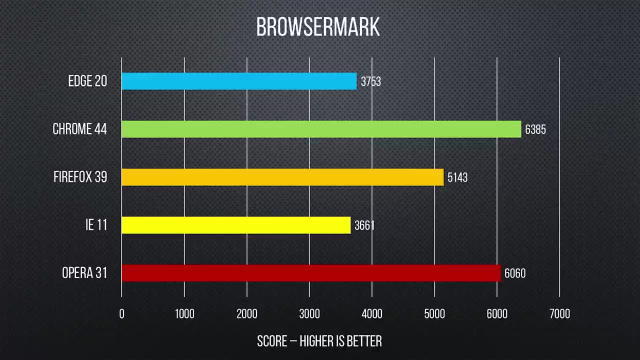 with all the latest versions of all browsers running vanilla without extensions, to ensure a fair fight. First up is browser marketing. This is a benchmark which analyzes both the performance and standards compliance of a given browser. Here, Chrome and Opera- remember it's Chrome based- run away with the contest with an overall score of over 6,000 each. 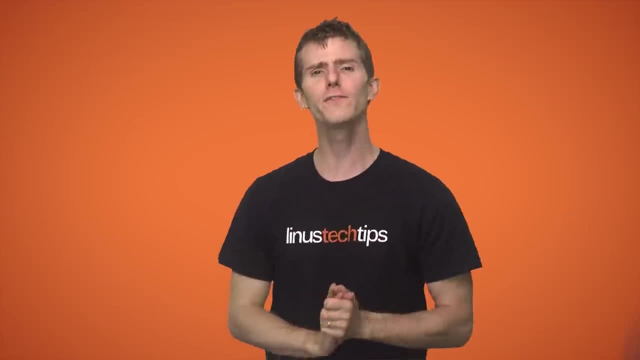 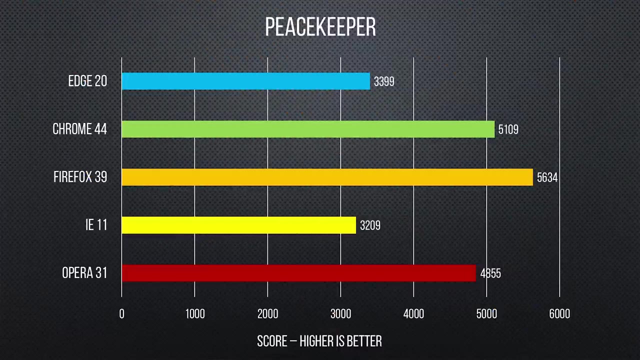 Both Edge and Internet Explorer 11 get crushed. Next is a variety of mostly JavaScript focused benchmarks, with some twists. Peacekeeper also looks at performance of a 2D game. WebExpert looks at HTML5 canvas performance And HTML5 test, as you can well imagine. 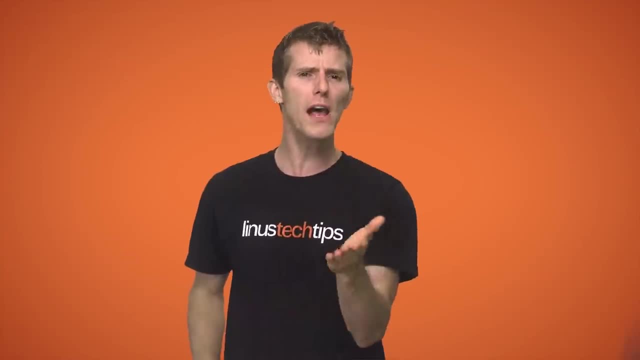 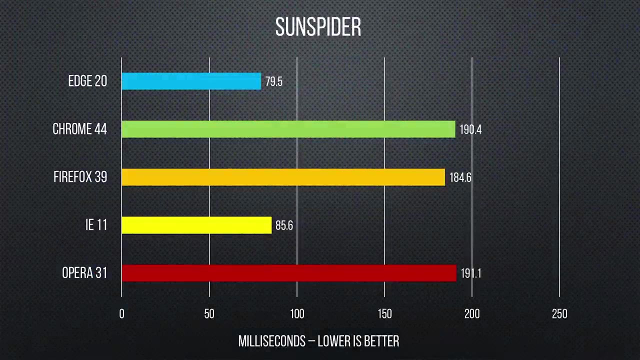 dials in on HTML5 performance, And this went pretty well overall, with Edge only being badly beaten in speedometer and HTML5 test and even pulling out victories in Sunspider and Jetstream. For our next test, we wanted to take a look at RAM usage. 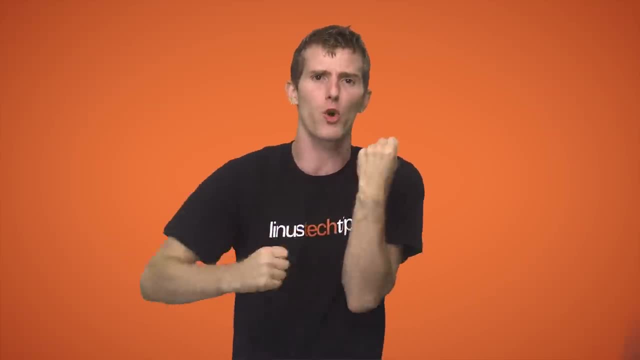 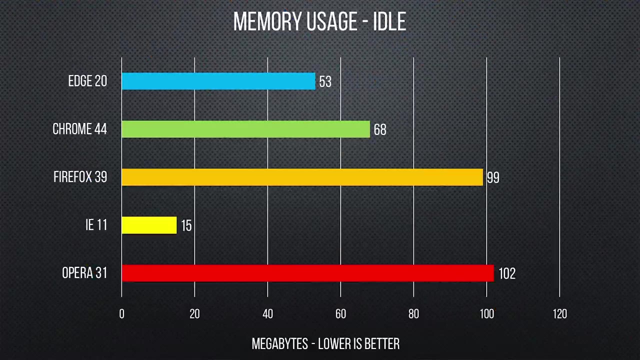 because, while it's all fine and good to talk about performance on a six core machine with 16 gigs of memory, not everyone is running a configuration like that. So, at idle, Internet Explorer 11 comes out on top, with Edge coming in second place. 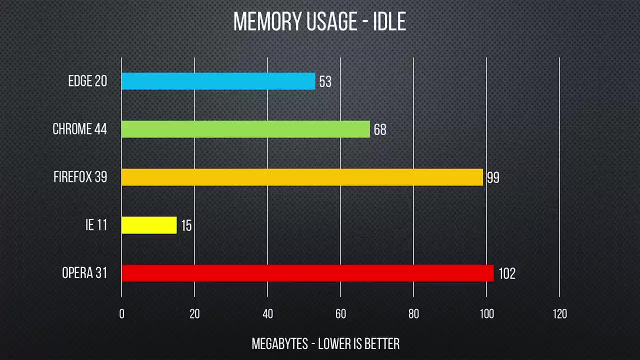 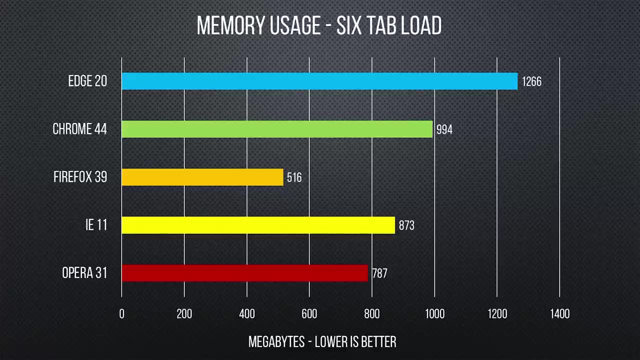 Then, under what I'd consider to be a fairly typical load, with an HD YouTube video playing Twitter and Facebook open, a long Wikipedia article loaded up somewhere else, the Amazon homepage and CNN homepage. Edge falls apart, managing even worse performance than our second last finisher, Chrome. 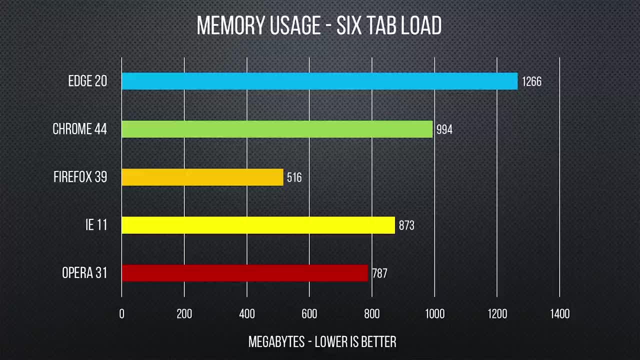 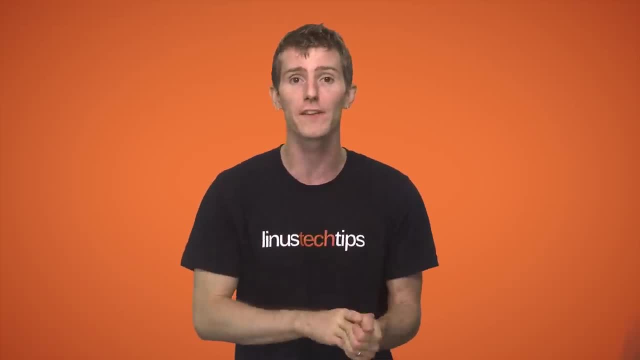 a browser that is well known for its RAM eating habits these days. We're not all about synthetics around here, though, so in our testing we also threw in some real world stuff, And John whipped out the high speed camera to do some practical web page loading tests. 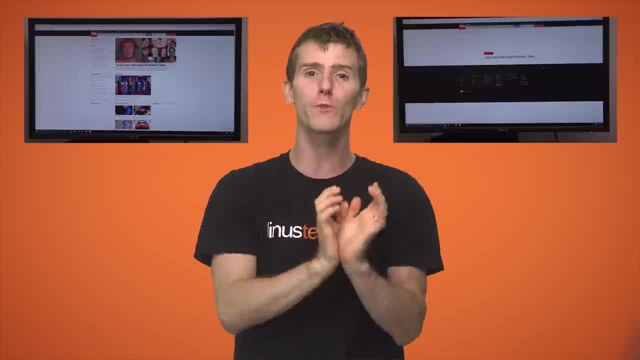 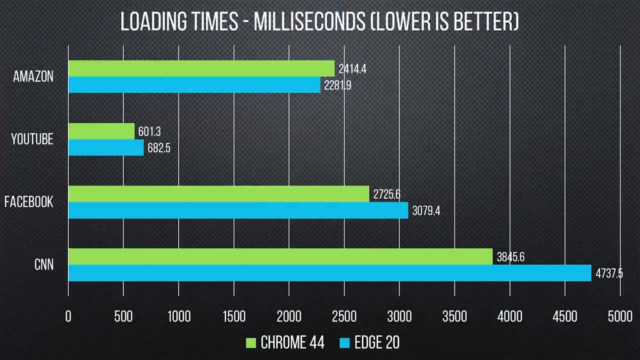 Edge was put up against Chrome side by side on our 200 megabit guaranteed fiber line and the results were measured by analyzing the footage to see how long the pages took to load For YouTube videos, Facebook and Amazon. I think it's safe to say that the difference was fairly negligible to a normal person. 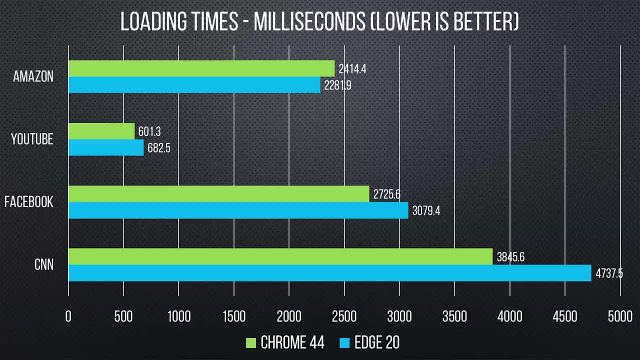 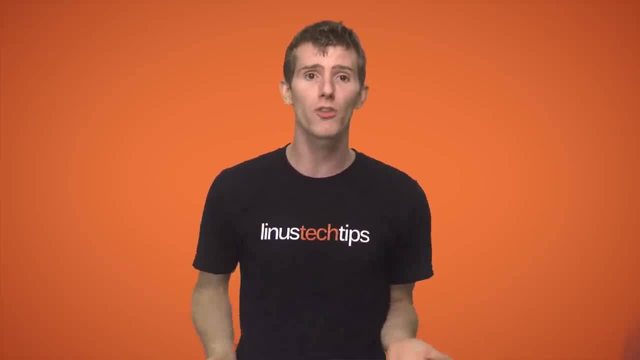 but for CNN. Edge got beaten by nearly a second Bummer. So the conclusion here is pretty straightforward: Edge isn't the fastest. It's the fastest browser out there, which no one, not even Microsoft, claimed it would be, And it still struggles with some compatibility issues. 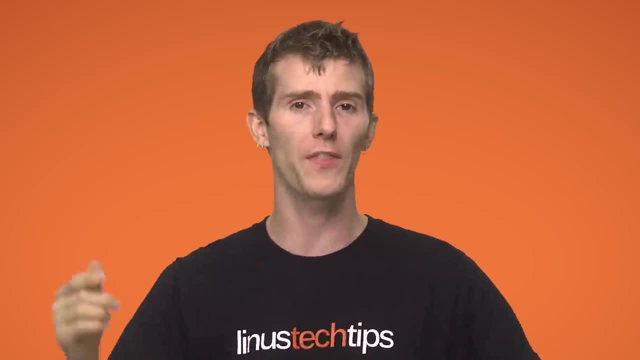 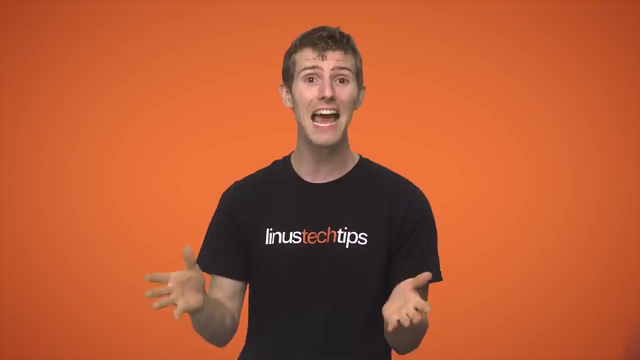 although that won't surprise you if you've read any of the user reviews out there on the net. But the good news is that it is a big leap forward compared to Internet Explorer 11, which came in last. in all but two of the benchmarks we ran.